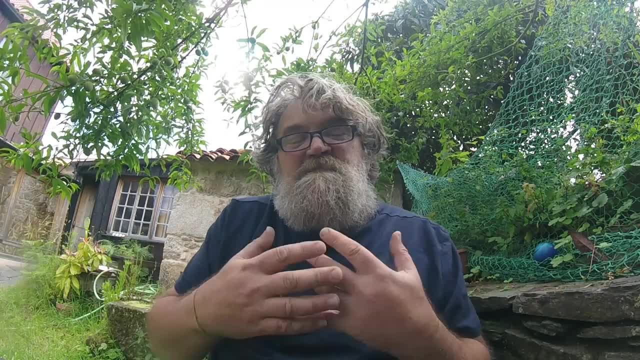 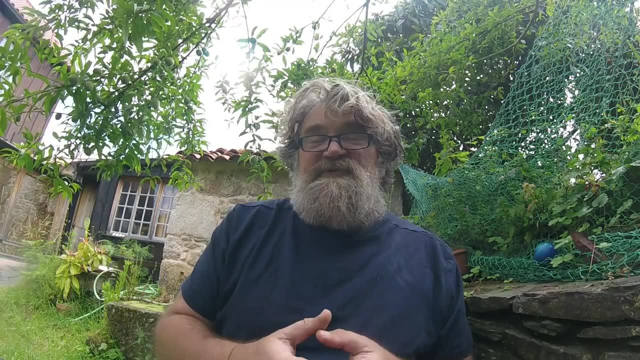 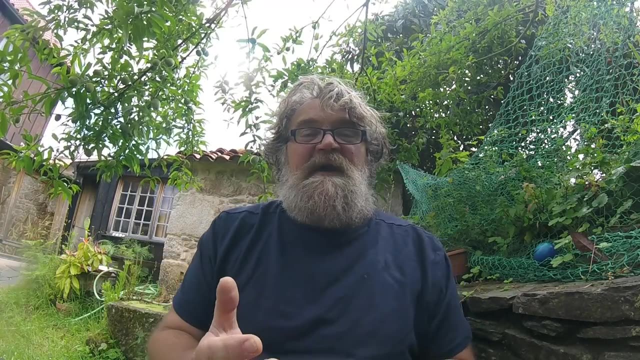 Okay, so burly. You could have a burly wrestler or a burly boxer. At a nightclub. a bouncer is pretty burly. He's a big guy, He's big and strong, A burly bodyguard, for example, as well. 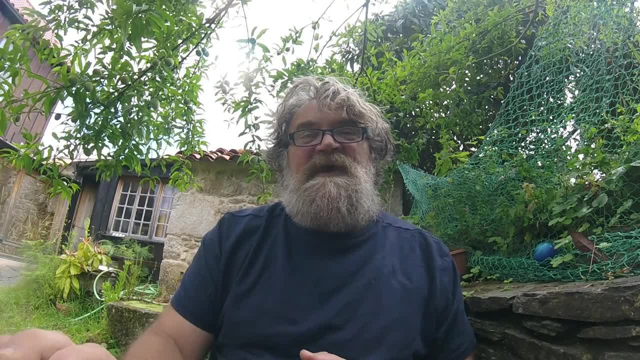 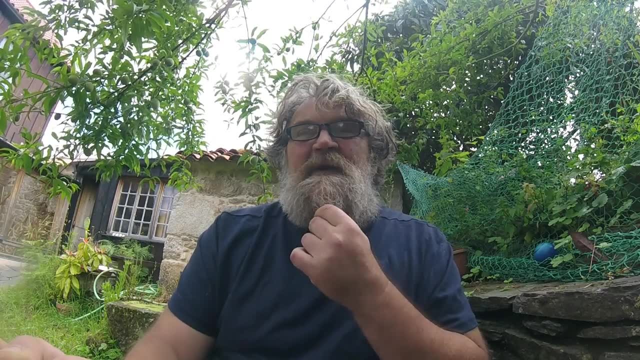 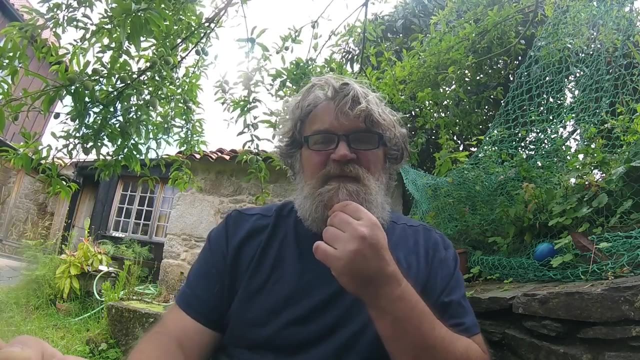 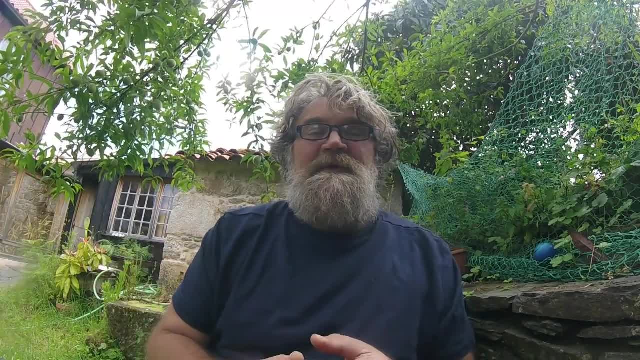 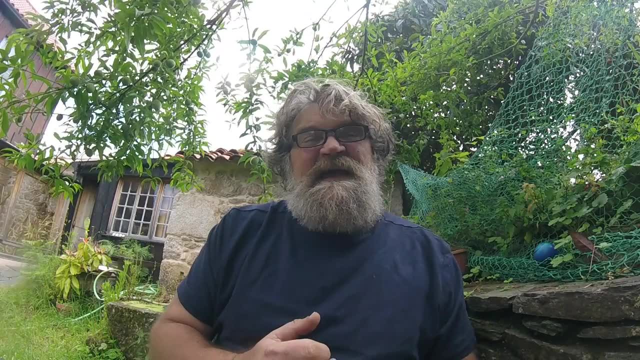 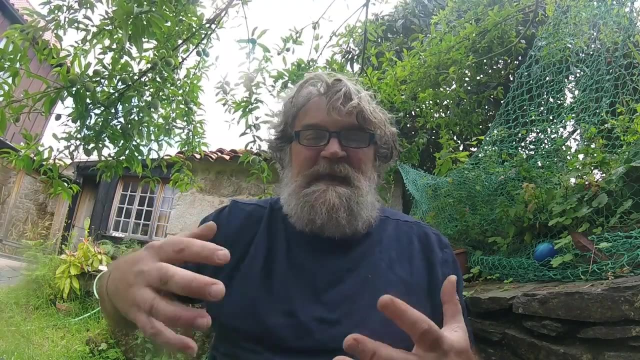 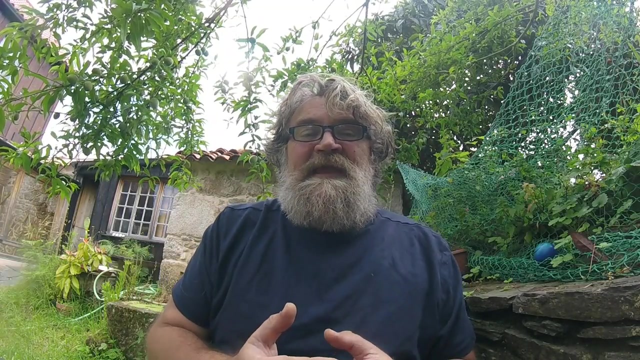 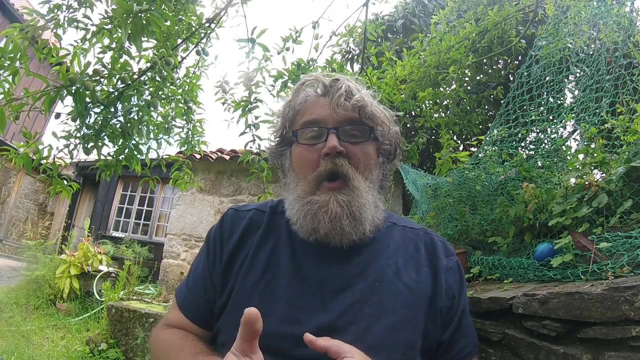 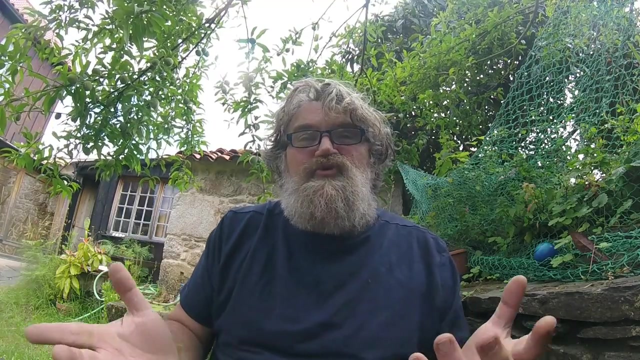 Okay, He's a big, burly bloke. Yeah, Heavily built, Well built, with everything about him's big, He's not fat, although he could be fattish, Yeah, But he's big as well. He's big all over, He's tall and he's not skinny. He's a great guy. So what about the origin of this? Well, this comes from Borlese, which is Old English, probably even Saxon, And it means built like a leader, built like a ruler, built like a king, And I guess in those days the leader had all the best things to do. Yeah, 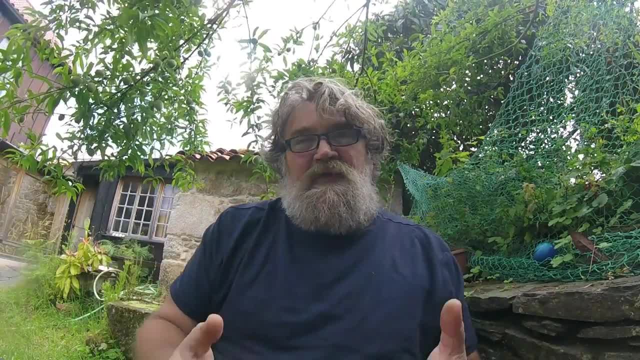 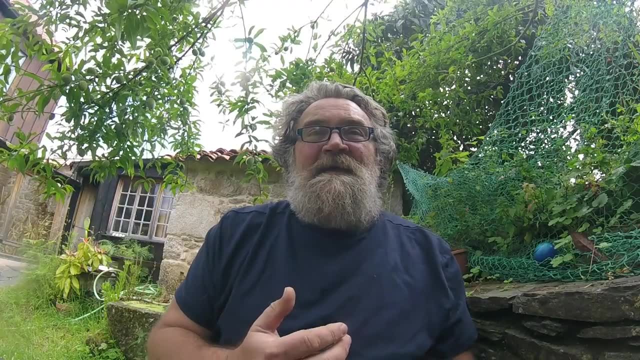 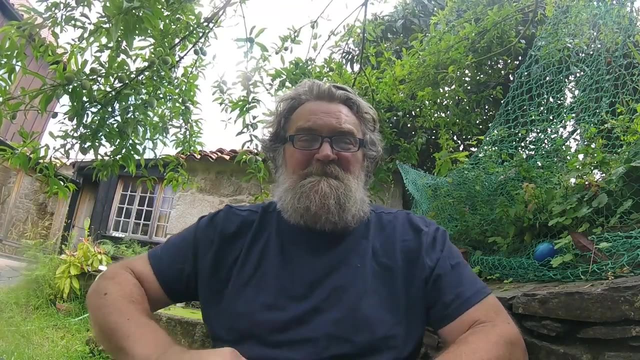 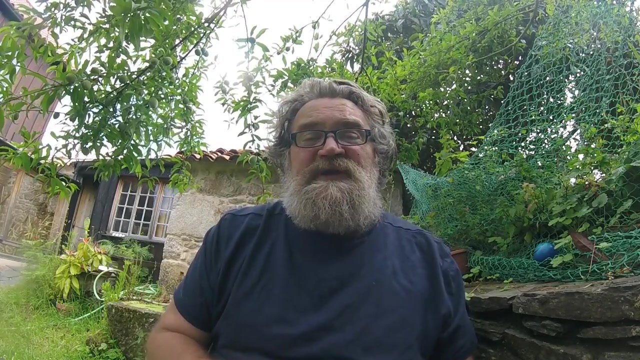 And he was normally a big chap. Well, he probably had to be a big chap as well to fight off anybody who was trying to kill him. Yeah, I think in those days, a leader needed to be a good warrior as well. Okay, So, burly, big and strong- Yeah, This would be a good word to use if you were writing an essay describing somebody. 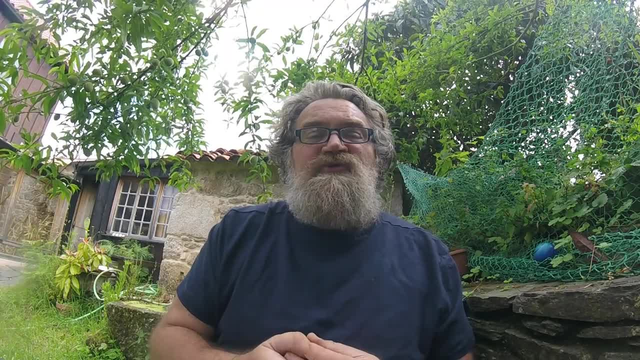 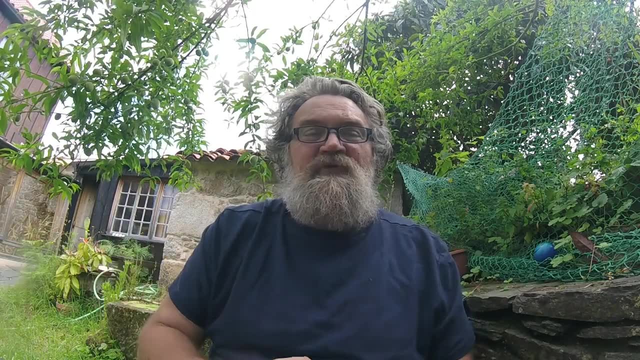 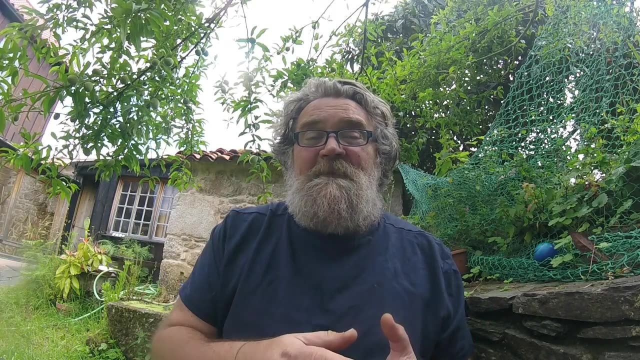 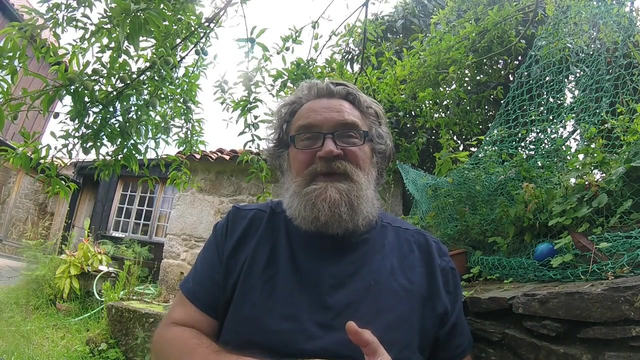